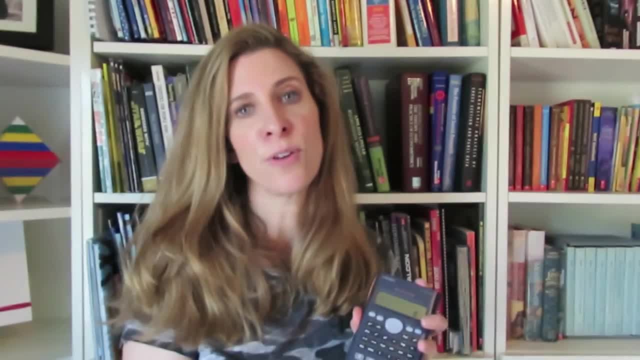 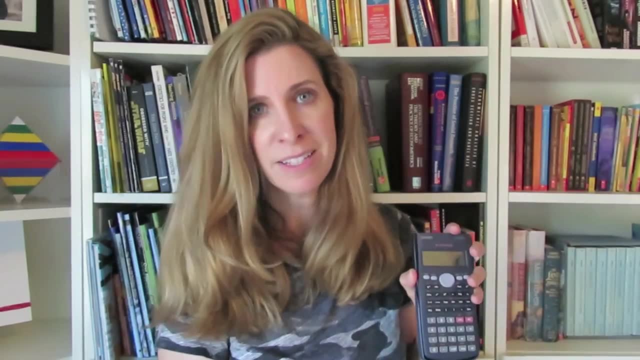 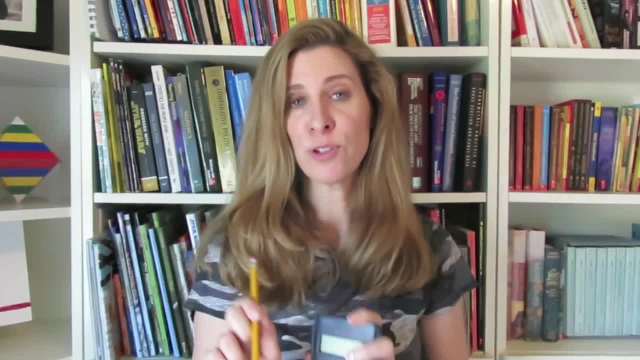 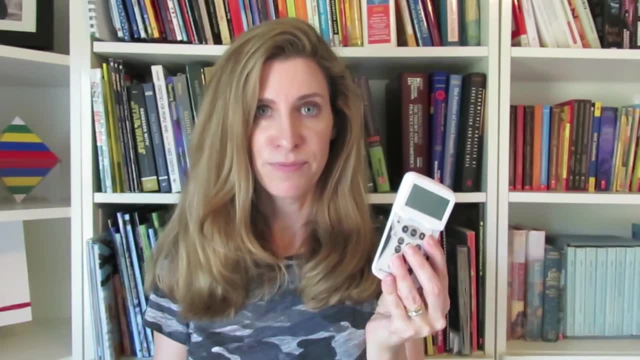 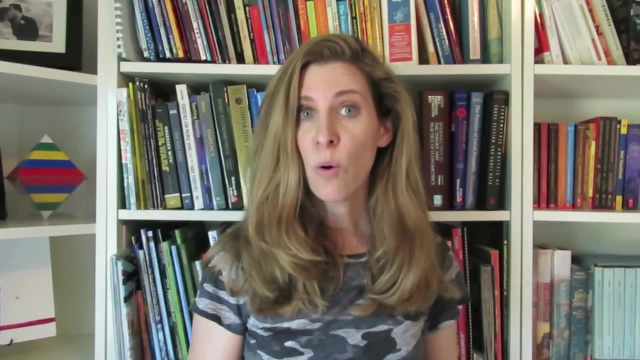 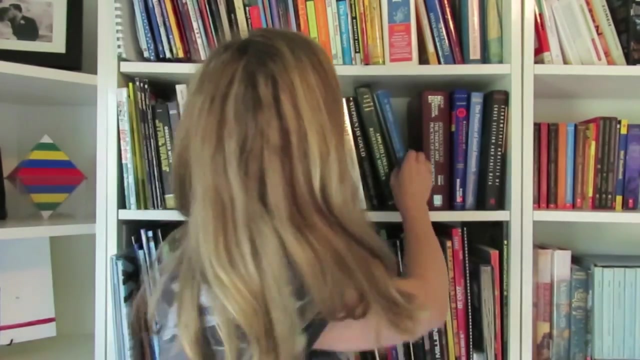 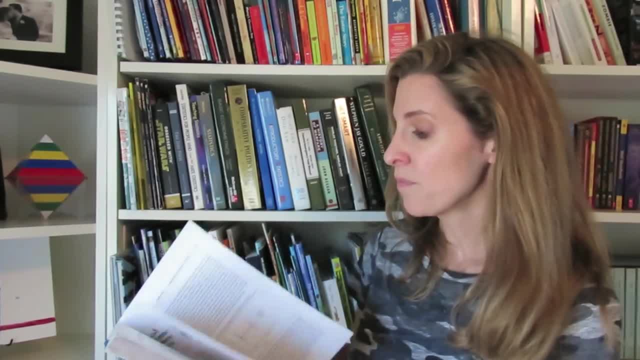 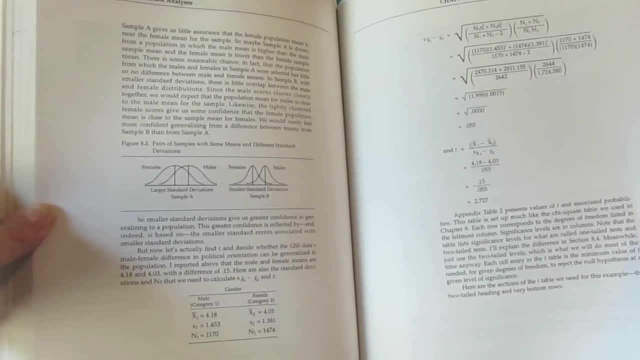 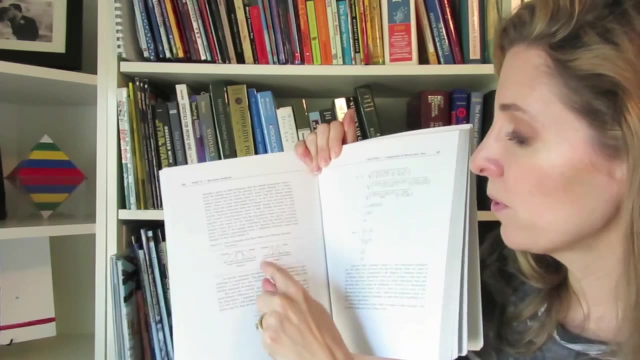 statistics course. It's a very, very accessible book, But what happens when you come to a page like this? What I find what most students do is they go read, read, read table. skip it, read, read, read. oh, small formula, skip it. another table, skip it. more formulas. 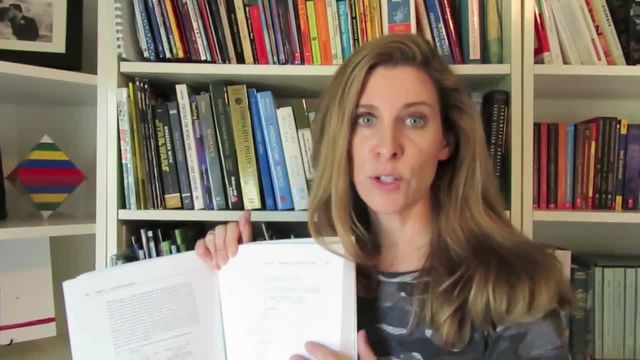 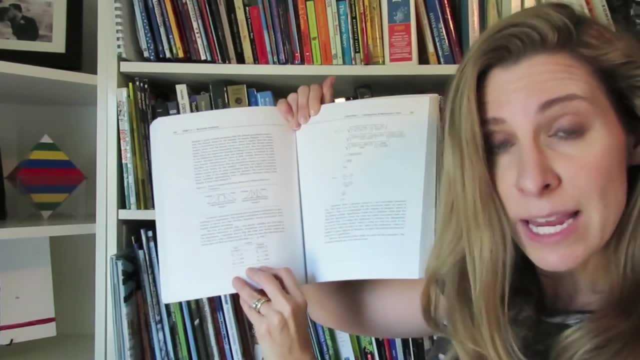 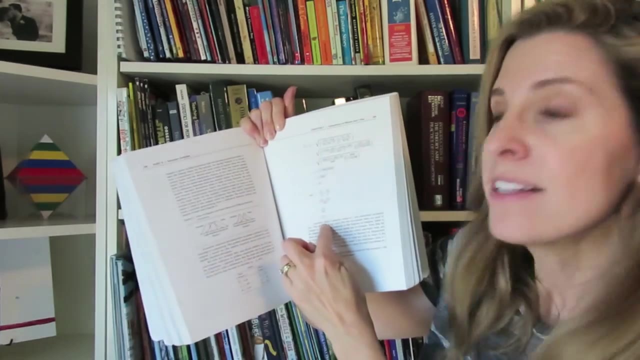 skip it Now. that is not how you read a statistics book. Every single mathematical formula must be read and understood. Every single table must be read and understood. You need to see where they get those numbers from. Can you figure out how these numbers have been calculated? That is how you read a. 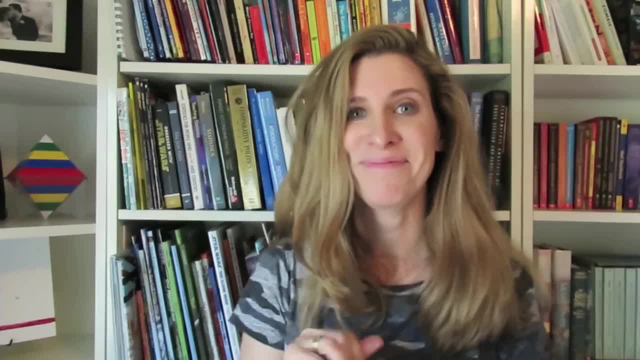 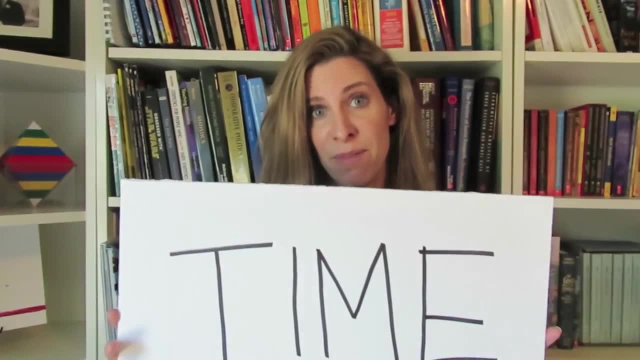 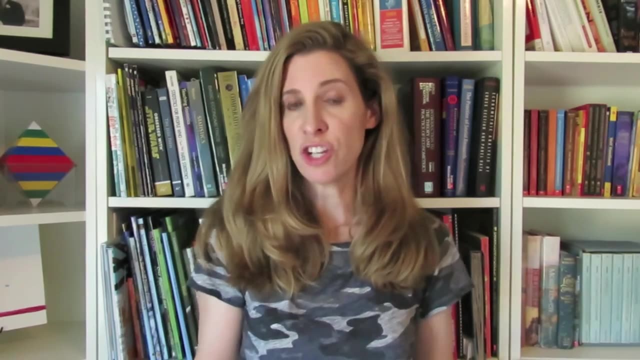 statistics book. The next important requirement for studying statistics successfully is math Time time. Now in my undergraduate courses, in the books that I assign maybe, I assign a chapter 20 to 30 pages a week. For my graduate courses likewise a. 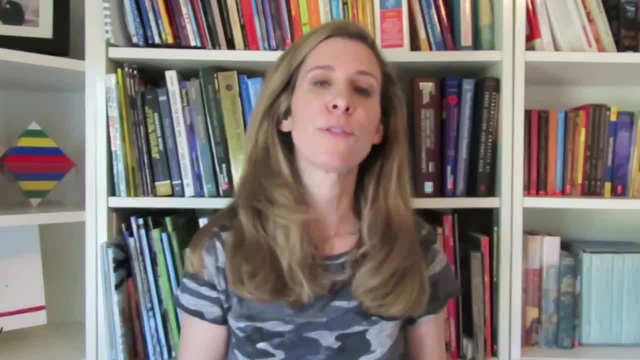 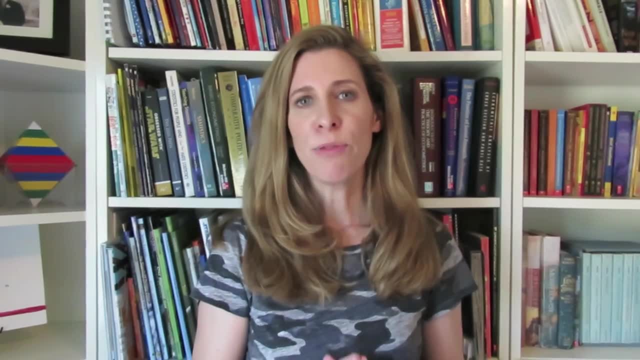 chapter a week is pretty much the average, with maybe a couple of supplementary articles. You know, maybe there you have, you know, 50 to 60 pages of reading a week. Now, that's not a lot of reading compared to what most professors. 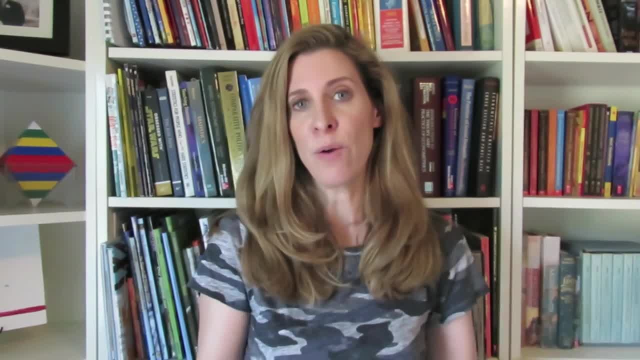 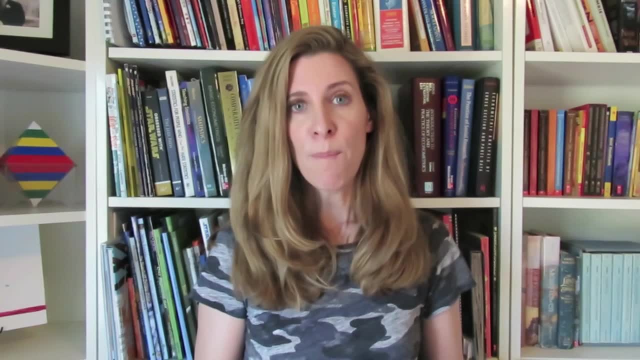 assign in the other classes What I assign, for example, in my Warren International Security class or my other graduate courses. it's maybe a third to a half of the amount of reading. But reading that amount of material should take you just as long, if not longer. 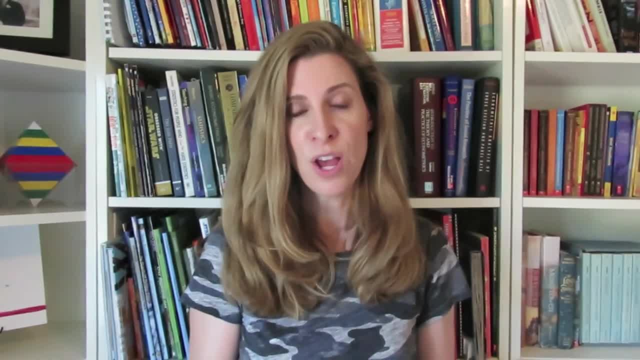 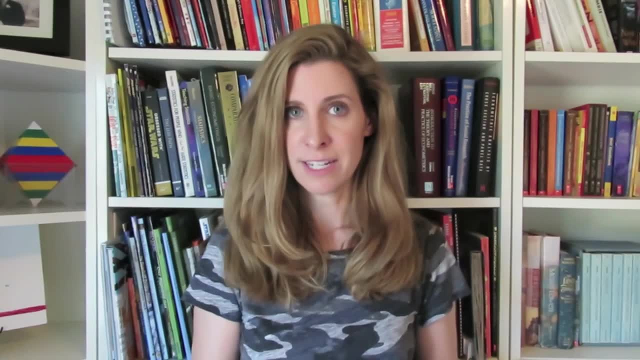 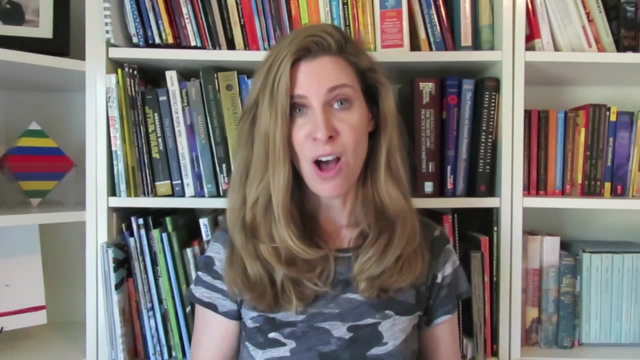 probably longer than the readings in your other courses. So don't be fooled by the short number of pages. It takes a long time to get through statistics material. Likewise, it takes a long time to get through statistics material to master the material. oftentimes students need to go through the same. 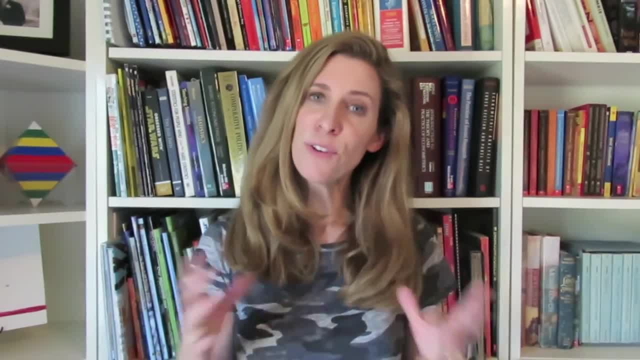 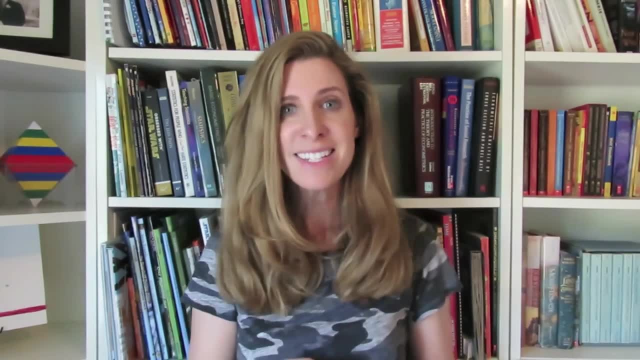 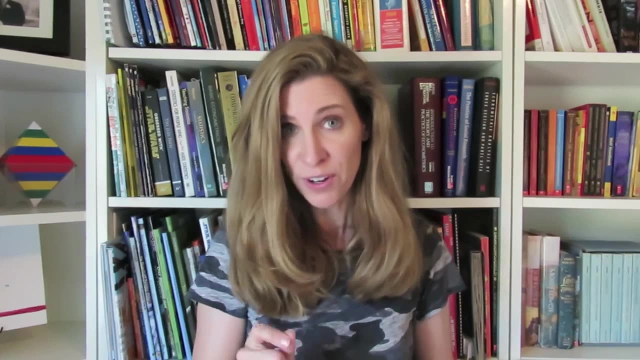 equations, the same problems several times. these are for even some of the very, very best students that I have in my courses. it's very rare where statistics comes very, very easily to a student, so don't be discouraged if you don't pick it up instantly. that's very, very difficult to do, but do expect to. 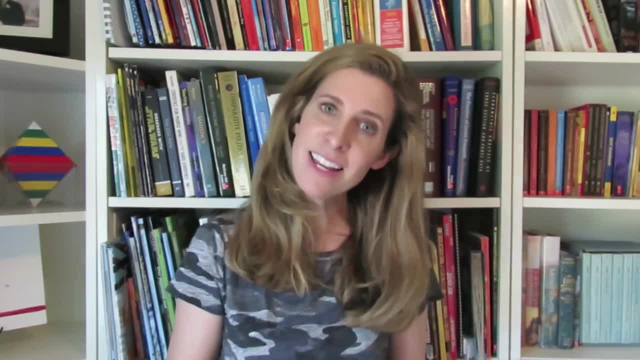 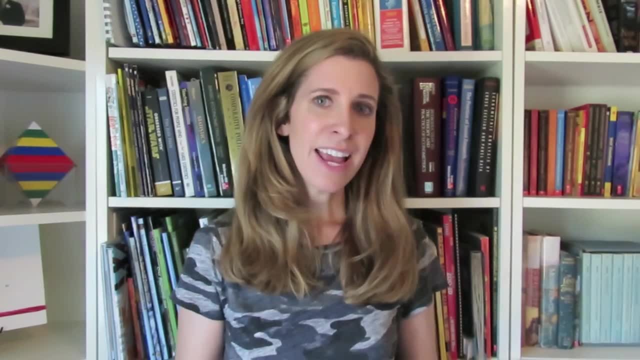 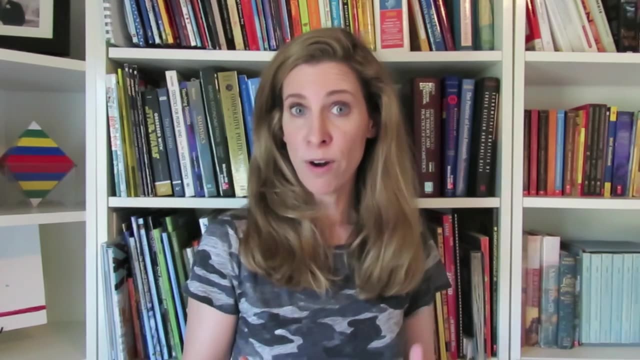 spend a significant amount of time in this class, as least as much, if not more, than in your other classes, and once you do, you will have statistics in your research toolbox forever. it's one of the most important tools that you can have as an informed citizen, as an educated human being on this planet and in this. 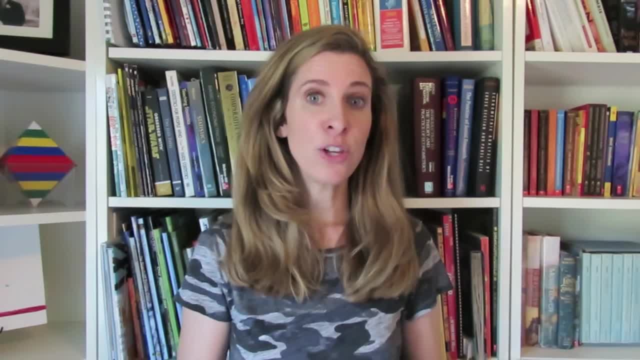 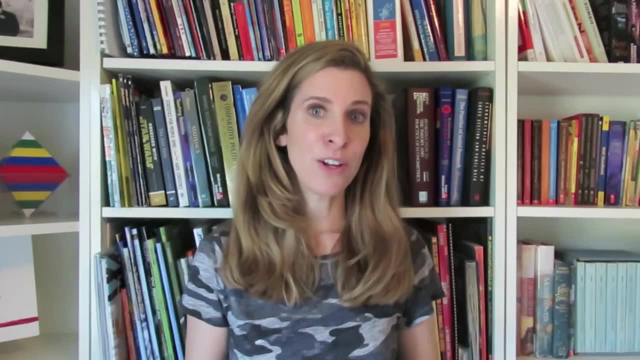 country and it's one of the, as well the most important things that you can put on your CV. so I hope this video has been helpful and I hope you enjoyed it. I hope this video was helpful and I hope it will inspire you to take the serious amount of. 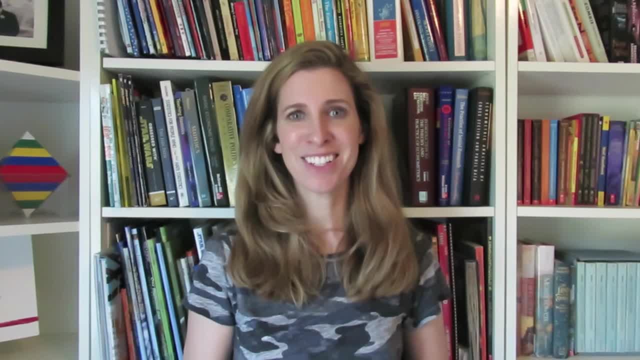 time it requires to study statistics successfully. 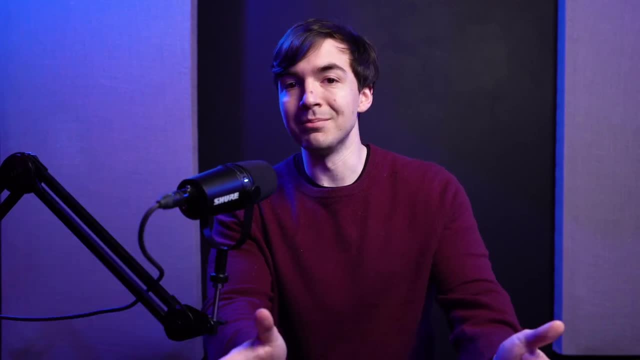 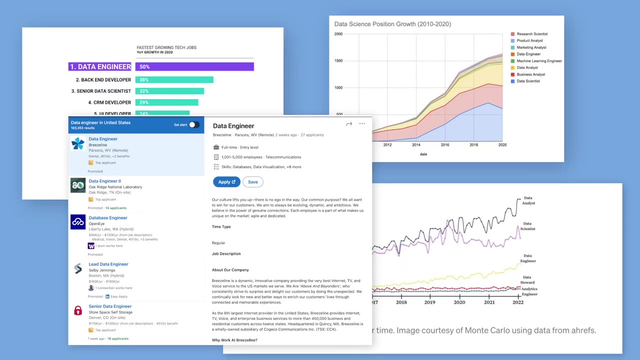 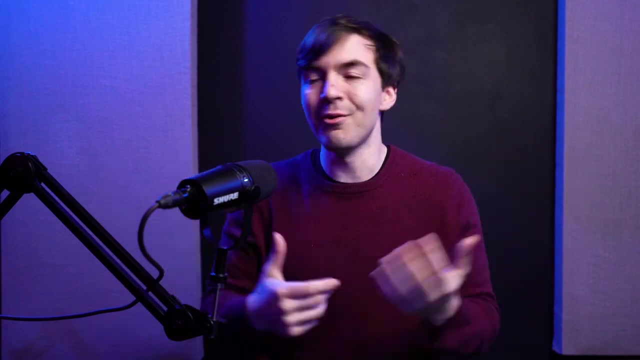 Data engineering continues to grow in terms of jobs. You can see this across multiple surveys and studies. I'm going to put a few up here from various people, kind of showing that there is increasing demand for people with data engineering skill sets. But if you're like me and you just got out of college, you had no idea what the term data engineering was or what they do. 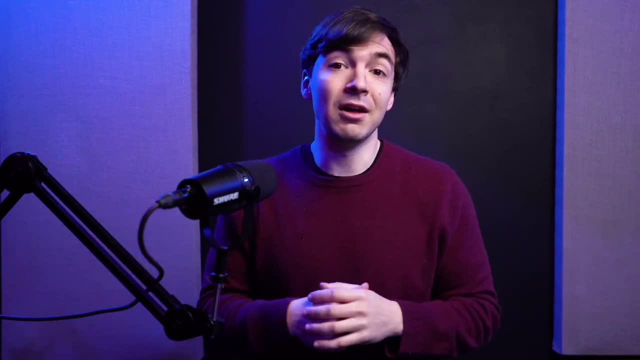 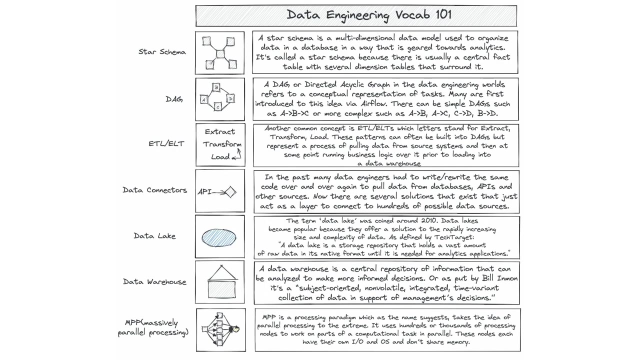 If you look across all the videos, including my own, you'll see lots of technologies. You'll see lots of tools. You'll hear words like data warehouse, data lake, ETL and a whole bunch of other stuff And maybe you get confused and think that's what data engineering is.